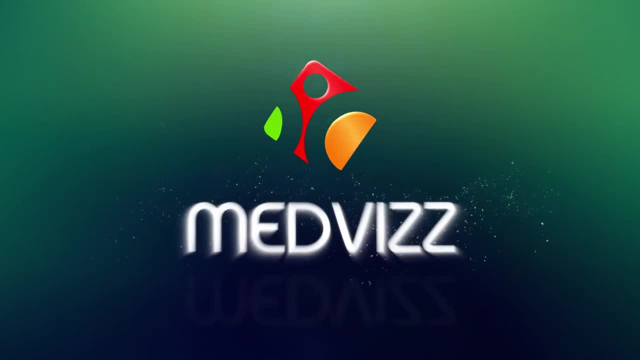 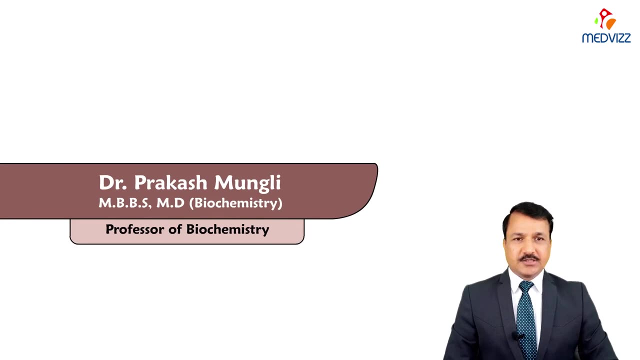 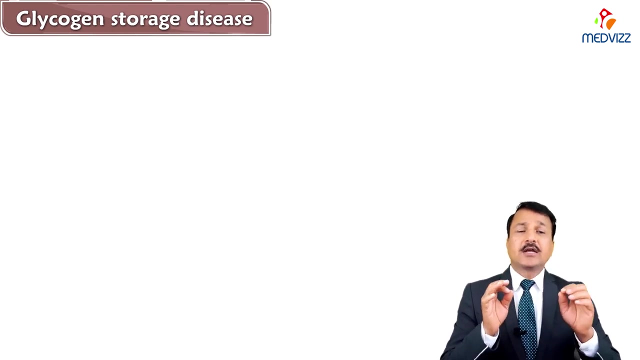 Hey everyone, I am Dr Prakash Mungli, professor of biochemistry. In this video I am going to explain you all about glycogen storage disease type 1.. In that glycogen storage disease type 1a, that is, Von Gerke disease. Let's get into all the details of Von Gerke disease. So before I 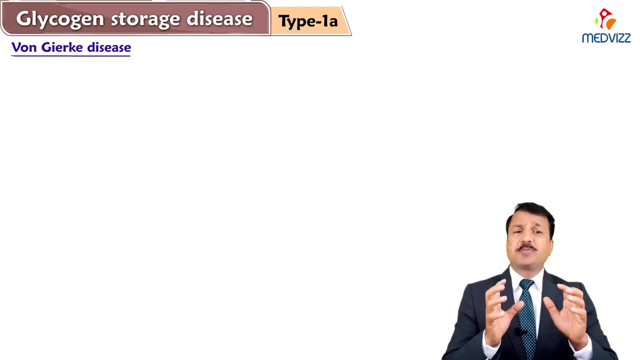 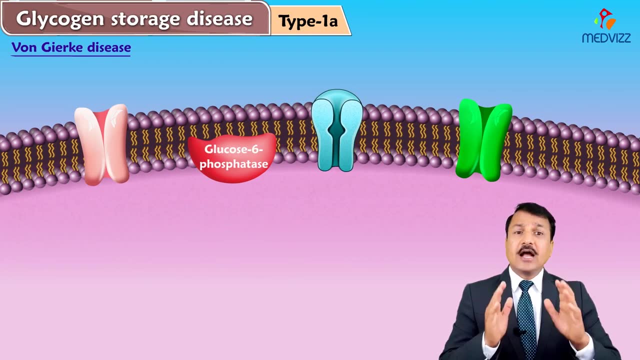 take you into Von Gerke disease. so I am going to briefly explain you what is the function of glucose 6-phosphatase enzyme, which is deficient in Von Gerke disease, and where it is located. So let's jump into little bit of that particular detail Now. glucose 6-phosphatase enzyme: it is 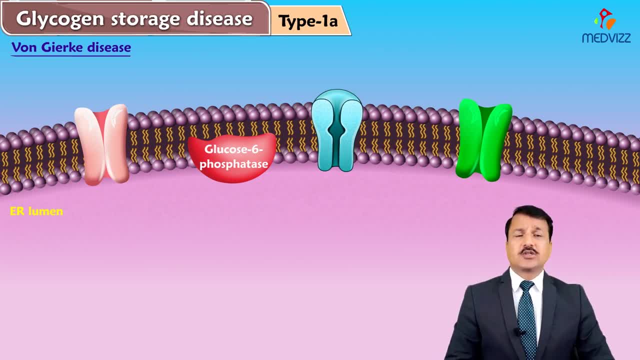 there in the lumen of the endoplasmic reticular, basically attached to the endoplasmic reticular membrane, towards the luminal side Now, whenever the glucose 6-phosphate has to be converted into glucose molecules. so generally this happens whenever we are in fasting condition. 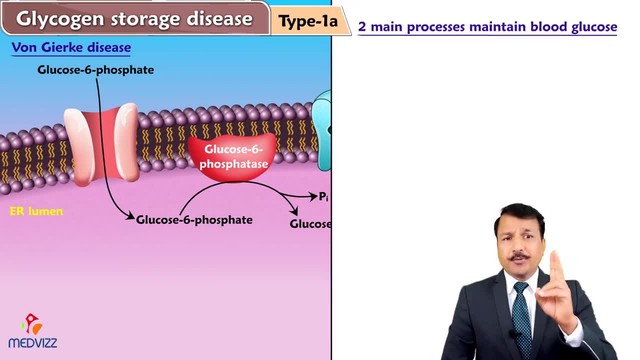 because when we go into fasting condition there are two processes that will help in maintenance of our blood glucose. One is gluconeogenesis, other is glycogen degradation. So when the glycogen degradation is going on, so the glycogen is broken down into glucose 1-phosphate in the 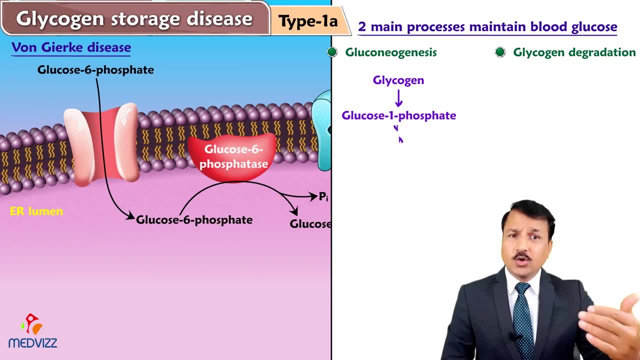 cytoplasm, This glucose 1-phosphate further converted into glucose 6-phosphate, and that glucose 6-phosphate acidifies, So it has to go into the lumen of the endoplasmic reticular to be converted into glucose, because 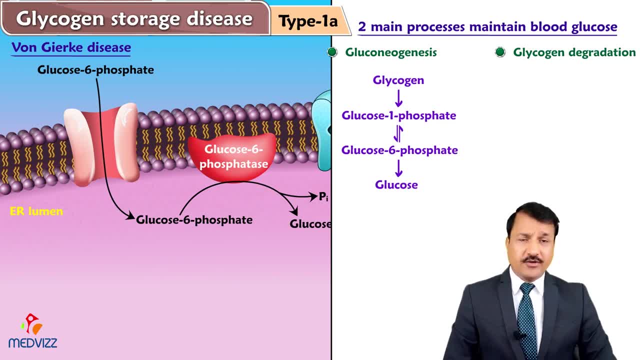 glucose 6-phosphatase enzyme. it is there in the lumen of endoplasmic reticular. Similarly for gluconeogenesis, when the non-carbohydrate sources like alanine, lactate, propionyl-CoA or glycerol, ultimately when they are converted into glucose 6-phosphate. glucose 6-phosphate. 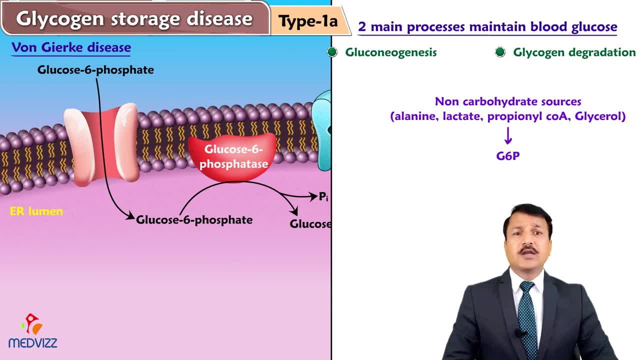 has to go into the lumen of endoplasmic reticular to be converted into glucose. So for both the glycogenesis and glycogen degradation you need glucose 6-phosphatase as the final enzyme and that is there in the lumen of endoplasmic reticular. That means glucose 6-phosphate has. 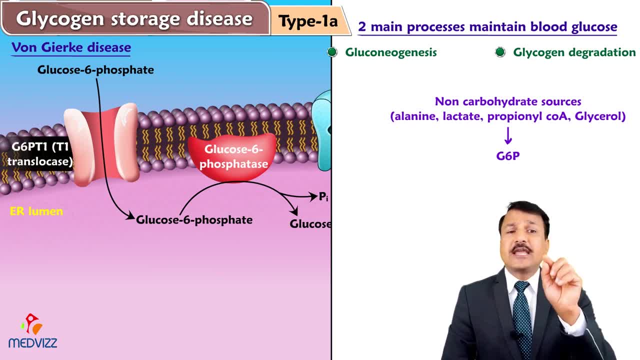 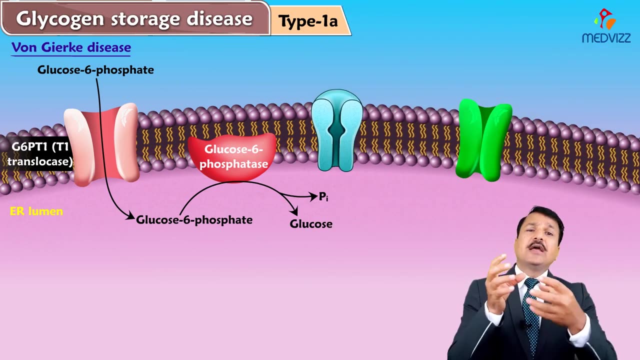 to go into the lumen of endoplasmic reticular and that needs T1-translocase protein. and once the T1-translocase protein allows this glucose 6-phosphate into the endoplasmic reticular- glucose 6-phosphatase enzyme, which is located in the endoplasmic reticular membrane- it is going to 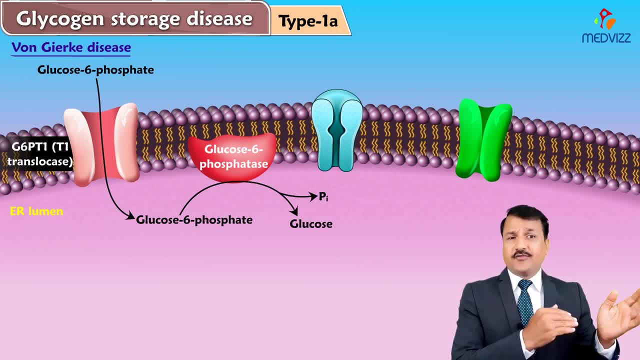 convert glucose 6-phosphate into glucose and inorganic phosphate released. and the inorganic phosphate comes out of the endoplasmic reticular into the cytoplasm by T2-translocase protein and the glucose comes out into the cytoplasm by T3-translocase protein. So like this: 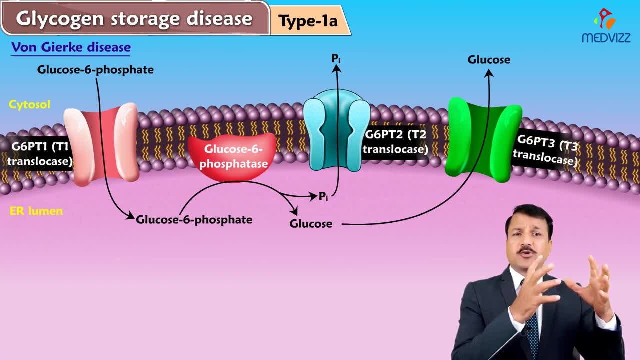 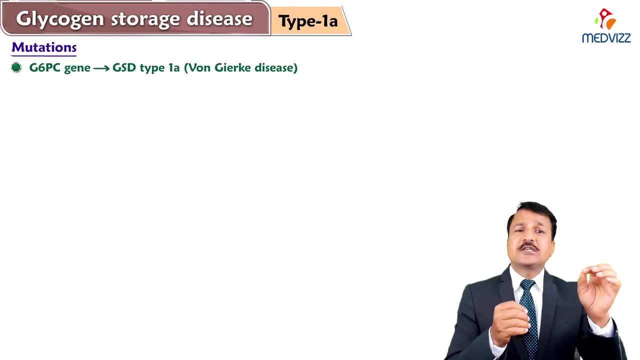 we need glucose 6-phosphatase, we need T1-translocase protein, T2-translocase protein and T3-translocase protein. So if there is a mutation in a gene called G6PC gene, which is coding for glucose 6-phosphatase enzyme, that will give rise to glycogen storage disease- type 1A. 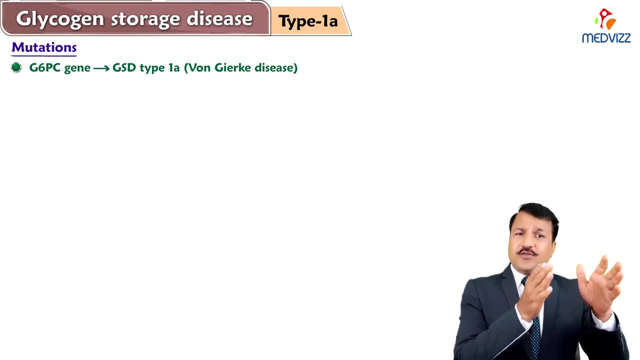 called Von-Gerke disease. Now, if there is a mutation in a gene coding for T1-translocase, that will give rise to glycogen storage disease type 1B. and similarly, although very rare so, if there is a mutation in T2-translocase that will give rise to glycogen storage disease type 1C. 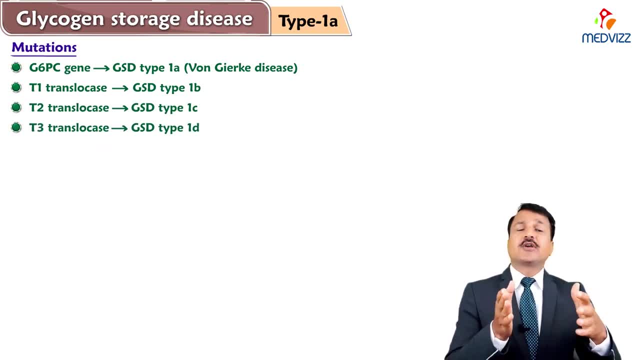 and if there is a mutation in T3-translocase that will give rise to glycogen storage disease type 1D. So, like this, there are 4 types of glycogen storage disorders: type 1A, 1B, 1C and 1D. 1A and. 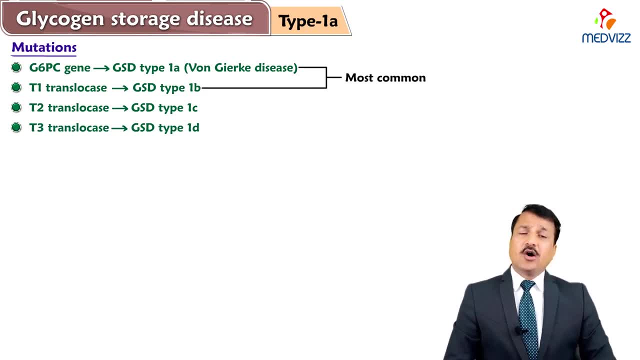 1B are the most common ones that are mentioned in the books. Now, out of this we are going to go into glycogen storage disease 1A and 1B. Now, in 1A there is a deficiency in glycogen storage. 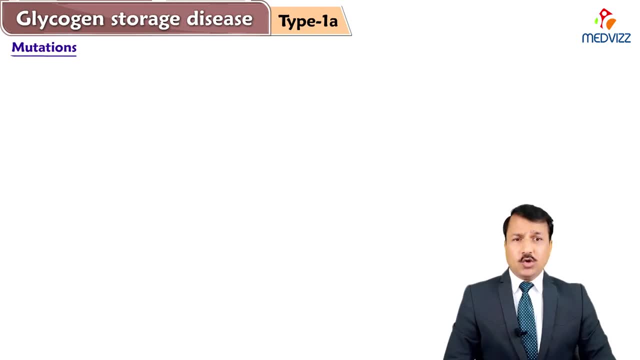 disease type 1A, there is a deficiency of glucose 6-phosphatase enzyme. So that means glucose 6-phosphate that comes from gluconeogenesis process or glycogen degradation under fasting condition. it simply accumulates in the cytoplasm because glucose 6-phosphatase enzyme is not available in 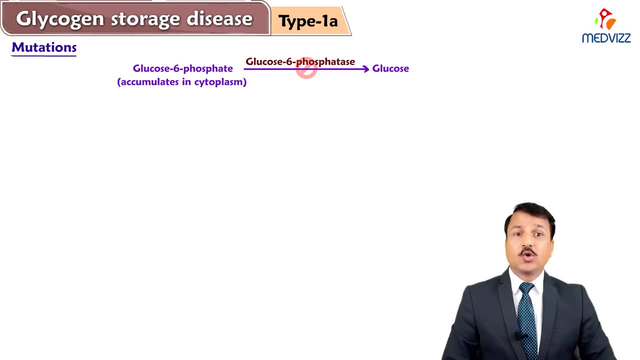 the endoplasmic reticulum or it is simply mutated. So what will happen to the glucose 6-phosphate in the cytoplasm? It simply builds up. It is not converted into glucose. So that means what happens Under fasting condition: the person will have fasting hypoglycemia because 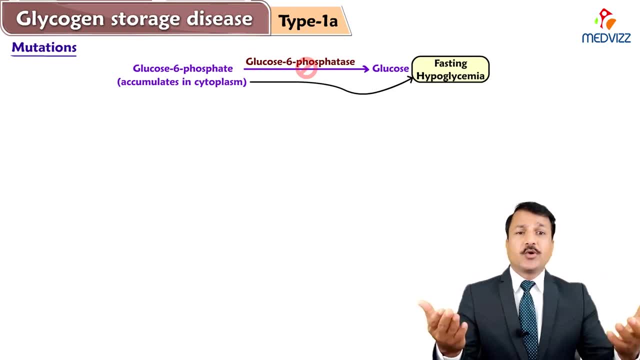 gluconeogenesis, glycogen degradation. both are not supporting to the maintenance of blood glucose because glucose 6-phosphatase enzyme is deficient. That is why a person will have fasting hypoglycemia, one of the important sign that you look for in Von Gerke disease. So that means 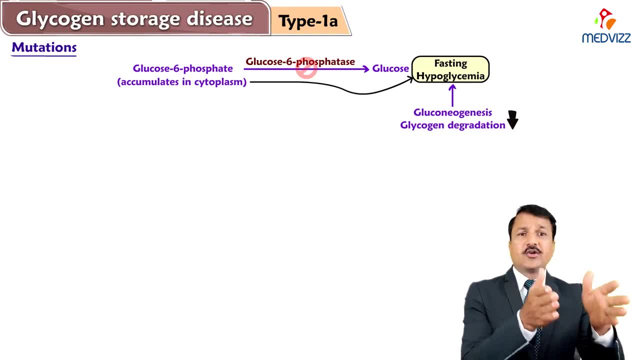 gluconeogenesis is down, glycogen degradation is down, fasting hypoglycemia is seen. and this fasting hypoglycemia, it will give rise to hypoglycemic seizures or hypochondriasis, Hypoglycemic convulsion. that is one of the sign you see in Von Gerke disease. Now then let us see. 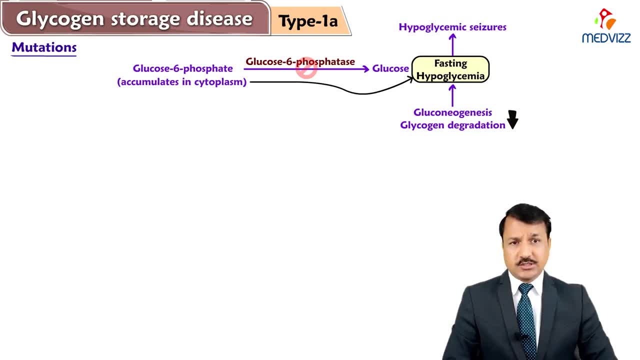 what happens to that? elevated levels, or accumulated glucose 6-phosphate. Now, this accumulated glucose 6-phosphate, it will be diverted into glycolysis in the cytoplasm, ultimately making pyruvate, and intermediate of the glycolysis is dihydroxystone phosphate. Now, what happens to the pyruvate? 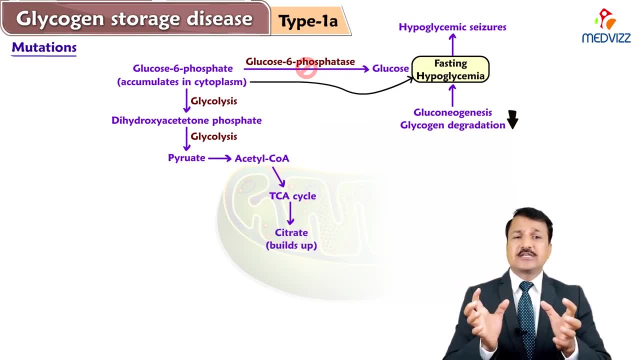 Cycle can go on initially, but when citrate builds up in the TCA cycle, citrate will move out of mitochondria into the cytoplasm and in the cytoplasm citrate breaks into acetyl-CoA and oxaloacetate. by citrate lyase enzyme and the acetyl-CoA. there it is diverted into fatty acid. 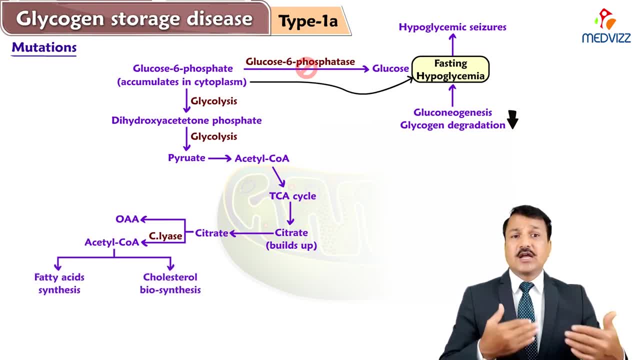 synthesis. it is diverted into cholesterol biosynthesis and the fatty acid can combine with glycerol 3-phosphate that can come from dihydroxystone phosphate. As I told you, dihydroxyacetone phosphate is one of the intermediate in the glycolysis process. 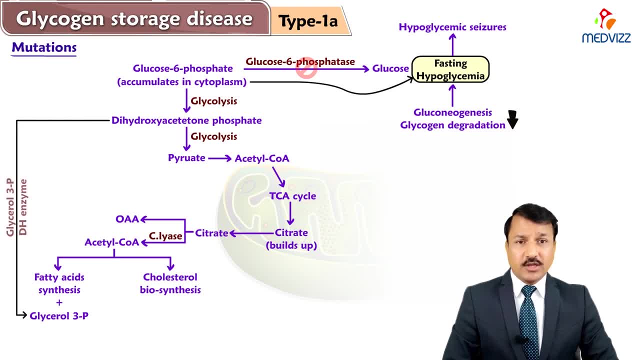 So dihydroxyacetone phosphate is converted to glycerol 3-phosphate in the endoplasmic reticulum by glycerol 3-phosphate dehydrogenase enzyme and that glycerol 3-phosphate it is acting as a. 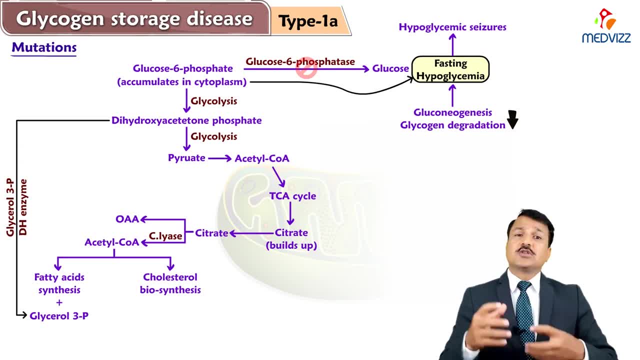 backbone for triacyl-glycerol synthesis. So the fatty acids coming from acetyl-CoA in the cytoplasm, which is basically coming from mitochondria as citrate, citrate converted to acetyl-CoA And acetyl-CoA is diverted into fatty acid. that fatty acid is esterified with glycerol. 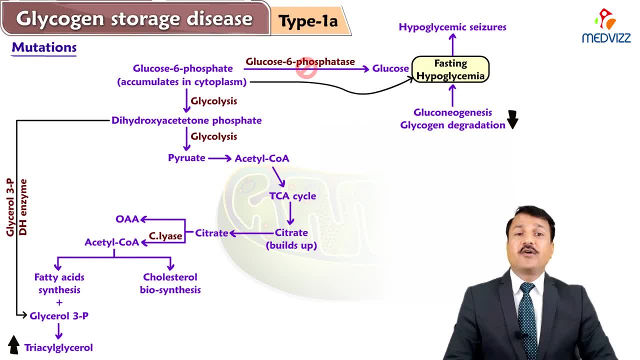 3-phosphate to make triacyl-glycerol. so there will be a buildup of triacyl-glycerol And then cholesterol, acetyl-CoA is diverted into cholesterol site. so cholesterol is a spotified with the fatty acid to make cholesterol ester in the endoplasmic reticulum. So cholesterol. 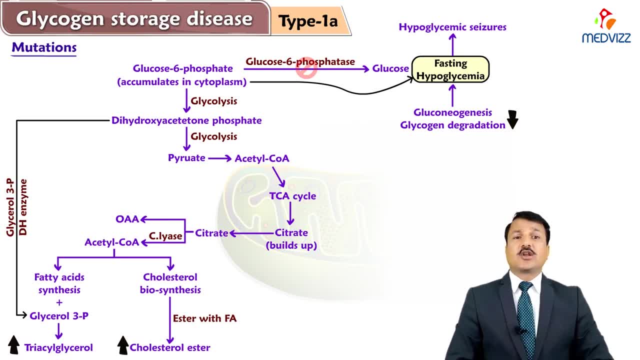 ester. so there is increasing triacyl-Glycerol, increasing cholesterol ester. all this will be getting into the blood, So زیادہ coh介 turns intoankur. examined as enzimothal uy Ралось. 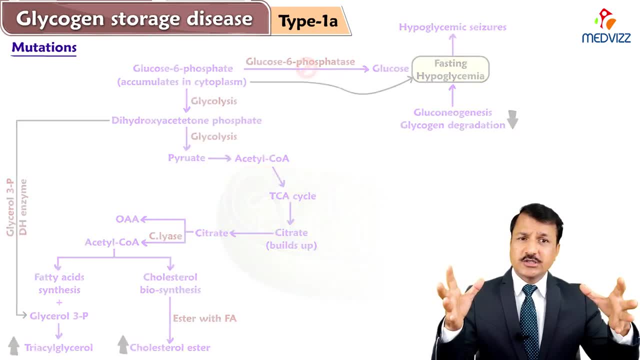 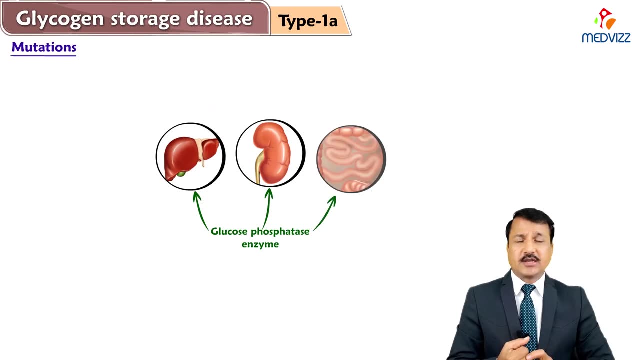 in the form of VLDL, because in the glucose 6-phosphatase enzyme it is located in three tissues, so mainly in the liver and then the kidney and in the small intestine. so what will happen? so the cholesterol ester and triacyl. 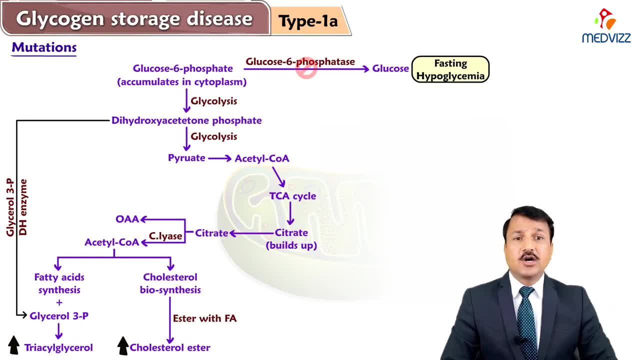 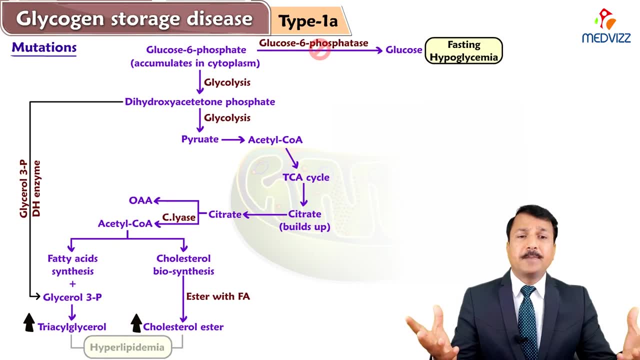 glycerol loaded VLDL, so they will be elevated in the blood. so I ultimately giving rise to hyper triacylglycerolemia and hypercholesterolemia. so overall it is hyperlipidemia condition and this hyperlipidemia is one of the important. 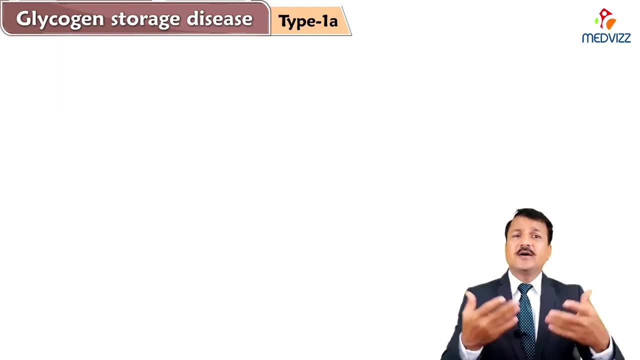 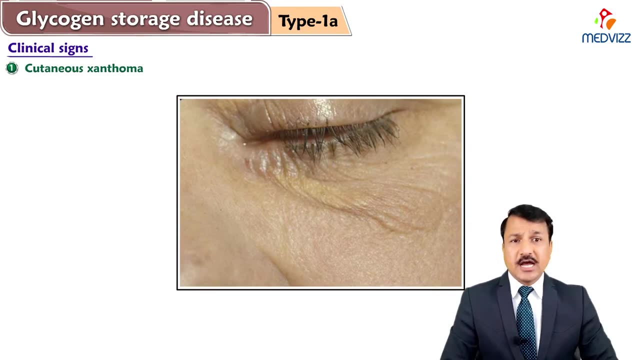 sign that we see in von Gerke disease and patients may show cutaneous xanthomas, so basically accumulation of fatty material beneath the skin. we call them as xanthomas. xanthomas is one of the sign we see in von Gerke disease and also von Gerke. patients will show basically the child with von Gerke. 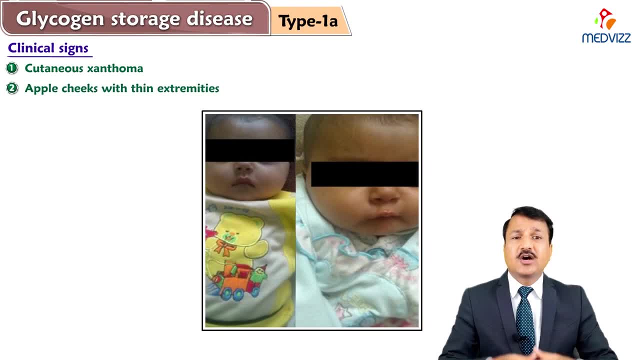 disease will show full cheeks, which is called as apple cheek or chubby cheeks. so, and the thin extremities. so it is a kind of abnormal fat distribution going on and these patients will show accumulation of glycogen in the liver, glycogen in the kidney. why? because elevated glucose 6-phosphate. it is positively acting on glycogen synthase. 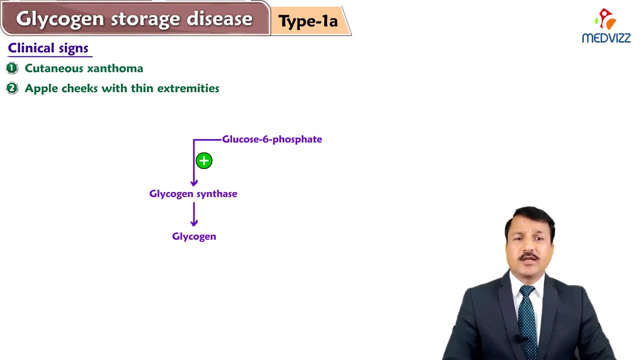 enzyme, because glucose 6-phosphate is a positive modulator on glycogen synthase. thereby, more and more glycogen is synthesized and glycogen degradation will be decreased. why? because same glucose 6-phosphate will have a negative effect on glycogen degradation enzyme called glycogen phosphorylase. 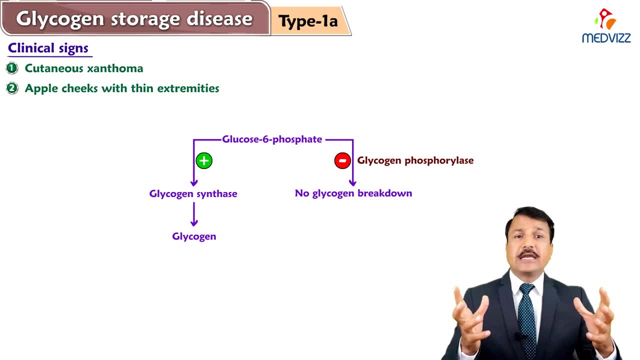 so thereby more glycogen is accumulated in the liver and kidney and that will give rise to hepatomegaly and renomegaly. and that's why in von Gerke patients we will see hepatoreno megaly. that will give rise to protuberant abdomen in 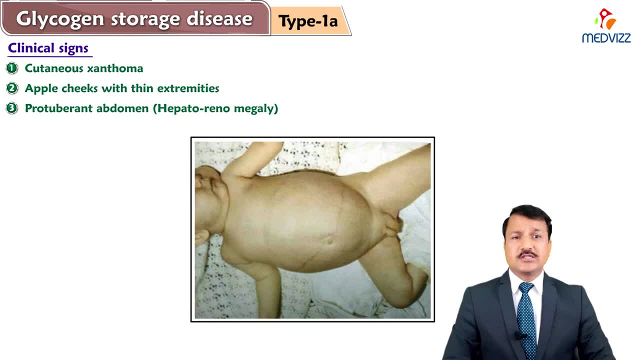 these patients. so that's why glycogen storage disease 1- it is referred as hepatorenal glycogenosis. now what are the other signs we are going to see here? so some of the pyruvate, other than going into acetyl CoA, is a. 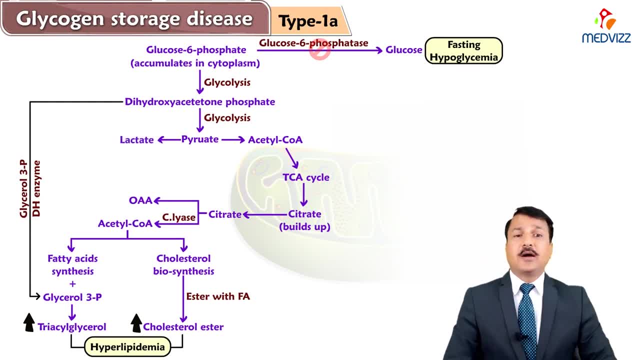 also diverted into lactate and there will be more lactate accumulated in the tissue, ultimately appearing in the blood, giving rise to lactic acidosis. so lactic acidosis eventually can give give rise to metabolic acidosis, along with the ketone bodies. why? because acetyl CoA can also be diverted into ketone bodies. 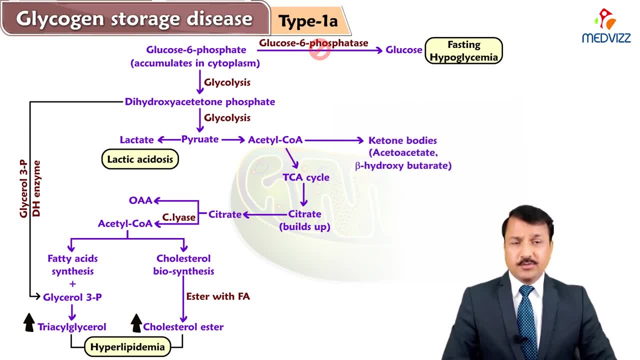 formation, that is, acetocetate and beta-hydroxybutyrate formation, and acetocetate, beta-hydroxybutyrate and lactate. all of them are acidic molecules. ultimately they will give rise to metabolic acidosis and the consequence of metabolic acidosis- one of the consequence- is hyperventilation. so 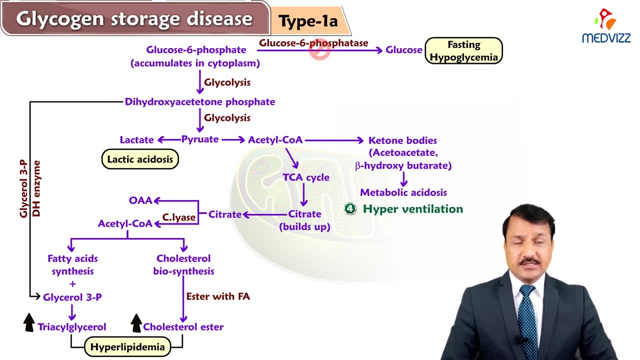 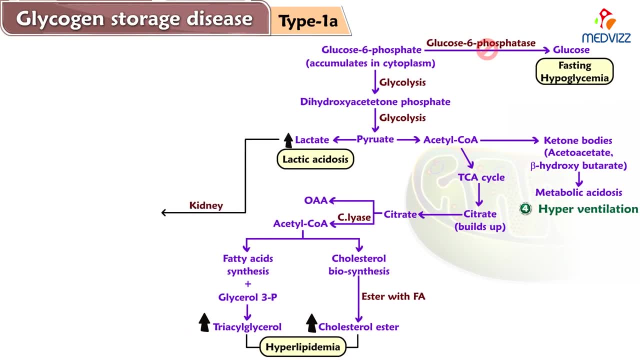 patients with von Gerke disease may show hyperventilation, one of the sign there now. so, since there is a lactic acidosis here, so lactate is elevated, note that in the kidney lactate is going to compete with the uric acid to make hyper. 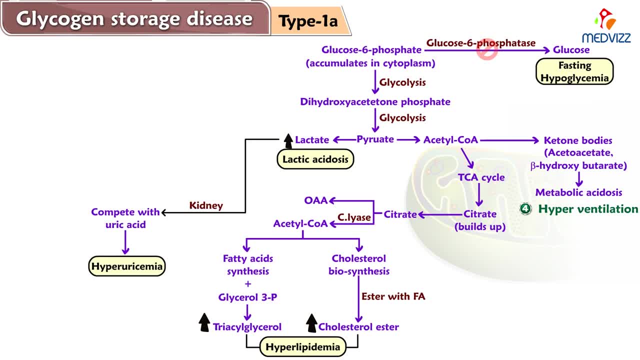 uricemia. so there'll be hyperuricemia, sign in von Gerke disease, and the hyperuricemia is, and the hyperuricemia will give rise to gouty arthritis because uric acid crystallizes in the joint space. So patient may show uric acid crystals in the joint space, giving rise to 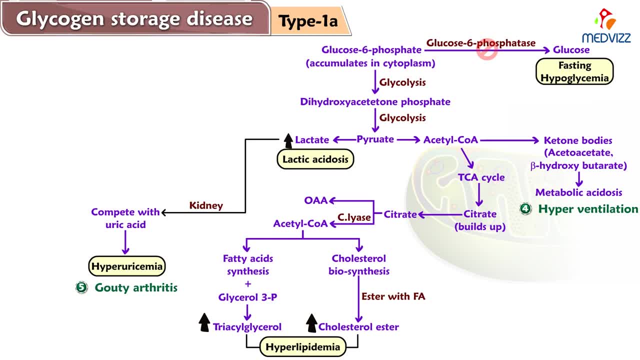 gouty arthritis or arthritis signs and symptoms, and also uric acid crystals can be seen in the urine also. So this is this is the other other, another important sign that you see, because of elevated lactate they're giving rise to hyperuricemia and then some of the glucose 6. 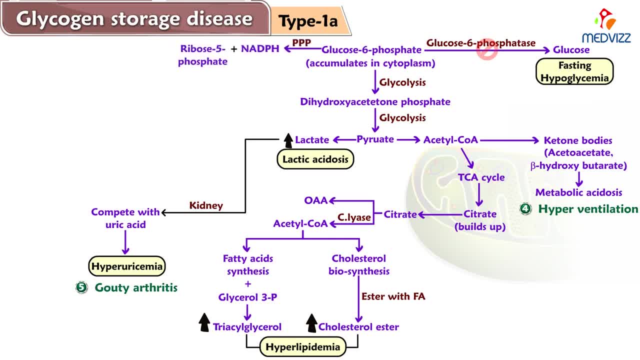 phosphate is diverted into pentose phosphate pathway, or HMP shunt, hexose monophosphate shunt. So in the pentose phosphate pathway. what happens? So more and more glucose 6 phosphate diverted into pentose phosphate pathway and that will give rise to increase in NADPHH plus and increase in. 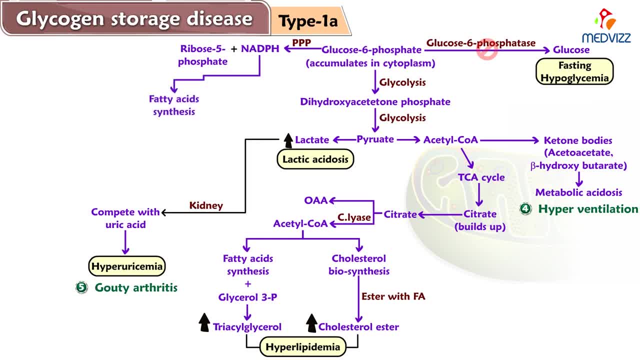 ribose 5 phosphate. So NADPHH plus is needed for fatty acid synthesis, cholesterol by synthesis. So it is supporting fatty acid synthesis and cholesterol synthesis, thereby increasing triglycerides, cholesterol esters, contributing, contributing to hyperlipidemia, which I have already explained to you. And what about ribose 5 phosphate? Ribose 5 phosphate is: 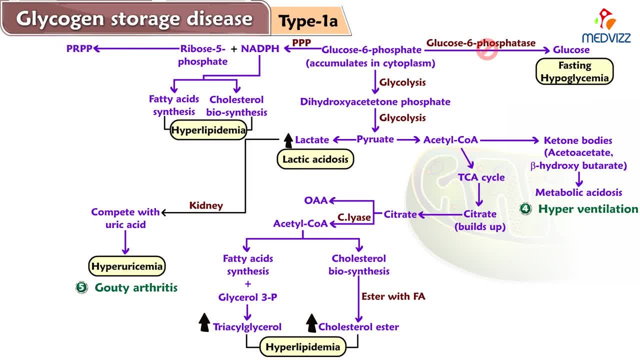 diverted into PRPP formation- phosphoribosyl pyrophosphate formation- and this PRPP is a positive modulator on purine nucleotide biosynthesis and pyrimidine nucleotide biosynthesis. So this is a positive modulator on purine nucleotide biosynthesis and pyrimidine. 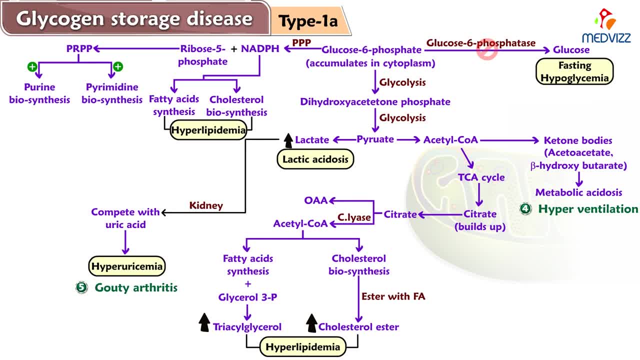 synthesis. So there will be increase in purine synthesis, increase in pyrimidine synthesis. So excess purines degradation. product of purine is uric acid, So that will also contribute to hyperuricemia that is seen in Von Gerke disease patient. So all these are the signs that we see. 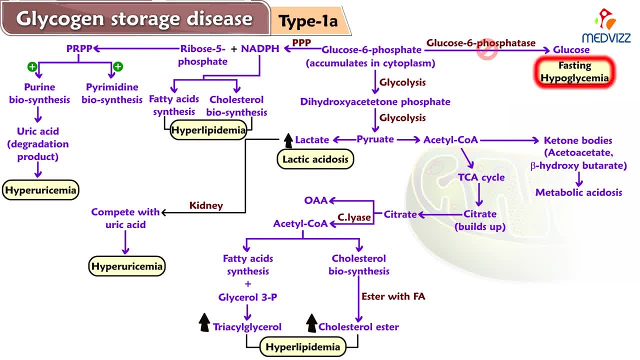 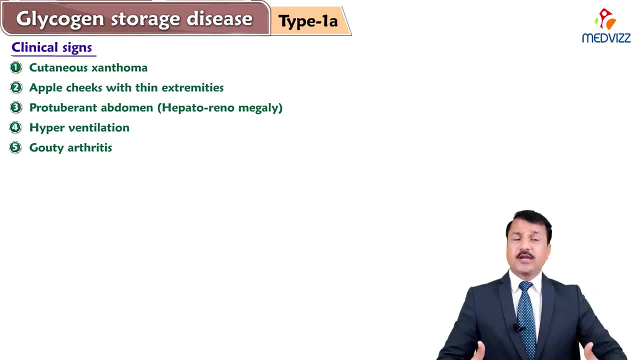 in Von Gerke disease patient. So what are the laboratory signs? Patient will show hypoglycemia under fasting condition, lactic acidosis, hyperlipidemia and ketoacidosis, hyperuricemia and hyperuricemia. Now what are the clinical signs and symptoms? So, patient will show protuburant. 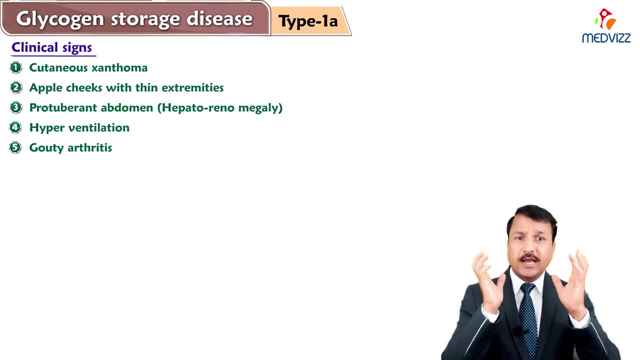 abdomen because of hepatorhinomegaly, full cheeks or apple cheeks, and cognitive impairment is seen in Von Gerke disease patients. So there will be thin extremities and then gouty arthritis signs and symptoms. xanthomas can be seen because of hyperlipidemia and metabolic acidosis giving rise. 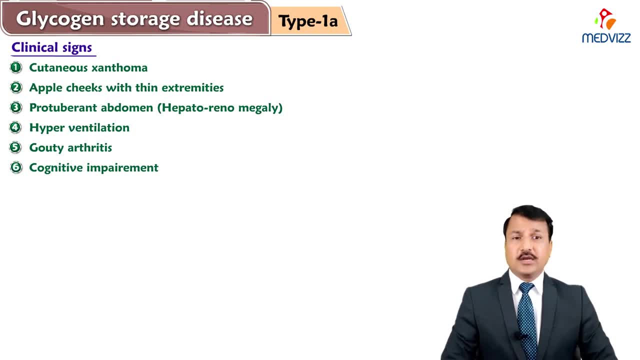 to hyperventilation signs. What is the treatment for Von Gerke disease? So, Von Gerke disease, before I go to the treatment. So let me explain you what is glycogen storage disease 1B? Glycogen storage disease 1B is: 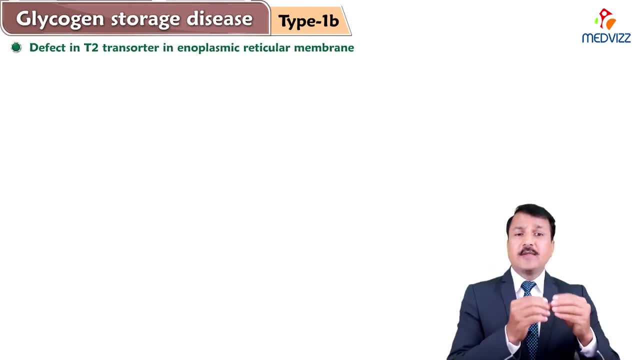 because of defect in T2 transporter in the endoplasmic reticular membrane. So that means glucose 6-phosphate is not entering into the lumina of endoplasmic reticulum. So signs and symptoms are very similar to Von Gerke disease, which I have explained. glycogen storage disease. 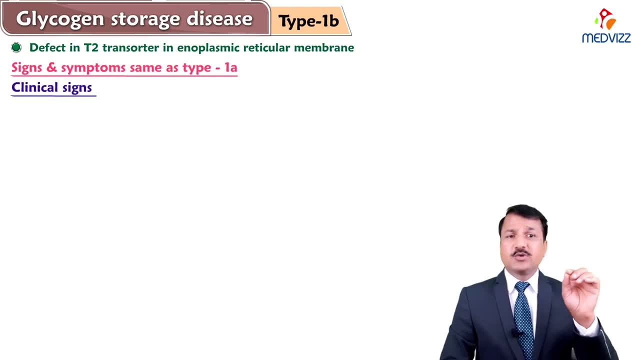 1A. Additionally type 1B patients will show neutropenia, neutrophil dysplasia, dysfunction, platelet impairment. All this will give rise to risk of bleeding, infection. risk of infection So, and patient may show frequent epistaxis. and all that bleeding in the nose and 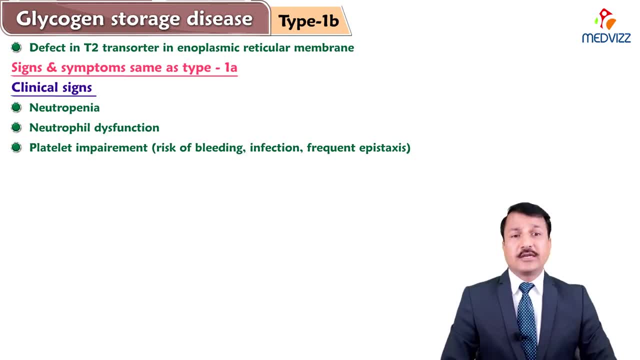 all, Though that's the additional sign, along with Von Gerke disease type 1A signs type 1B, as all these additional signs here. Now, what is the treatment for glycogen storage disease 1?? There is no specific treatment here. Gene therapy is under research, including chrysanthemum.